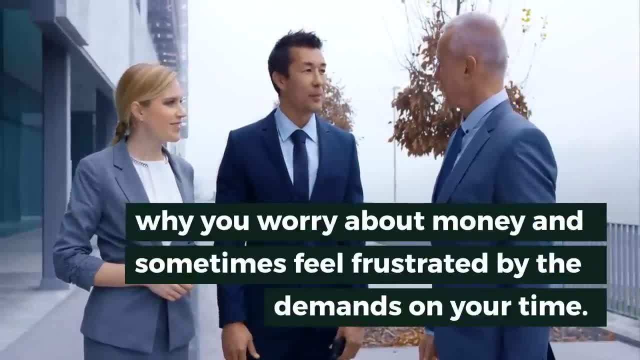 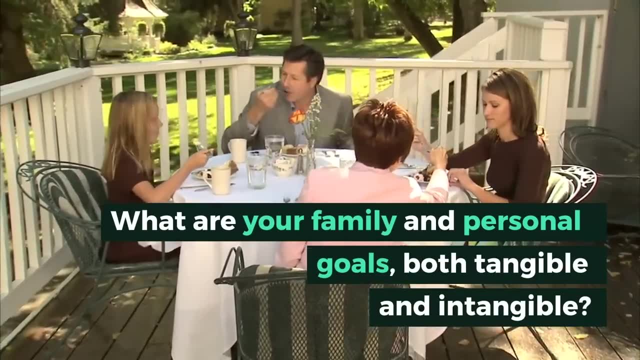 why you work hard and upgrade your skills, why you worry about money and sometimes feel frustrated by the demands on your time. What are your family and personal goals, Both tangible and intangible? A tangible family goal could be a bigger house, a better car. 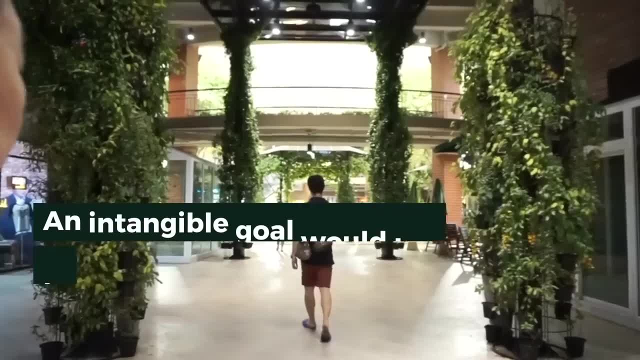 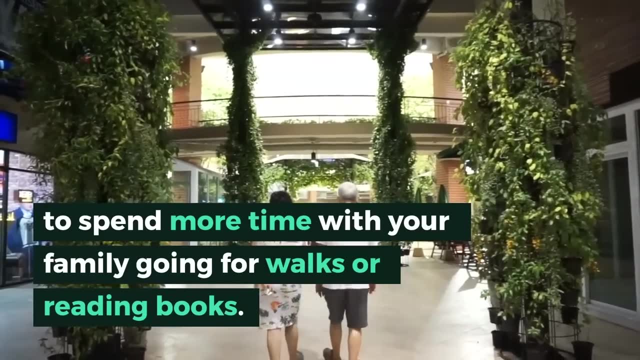 a larger television set, a vacation or anything else that costs money. goal would be to build a higher quality relationship with your spouse and children, to spend more time with your family, going for walks or reading books. achieving these family and personal goals are the real essence of time. 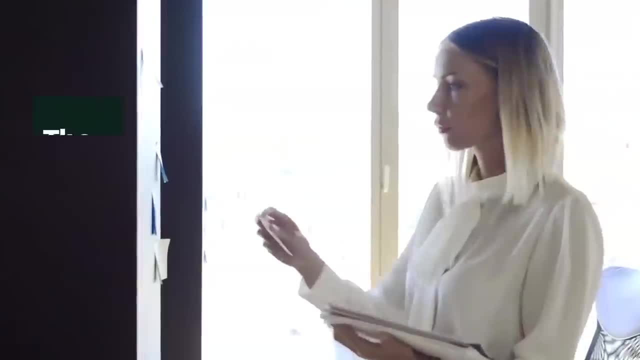 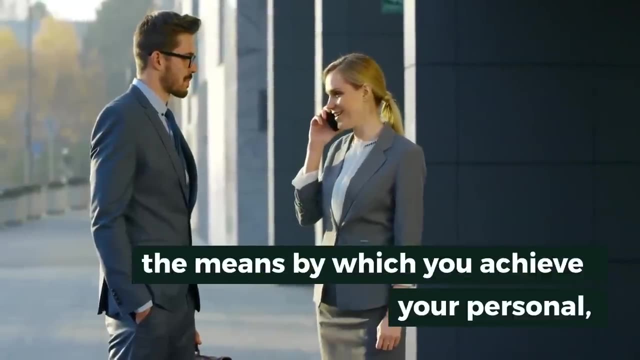 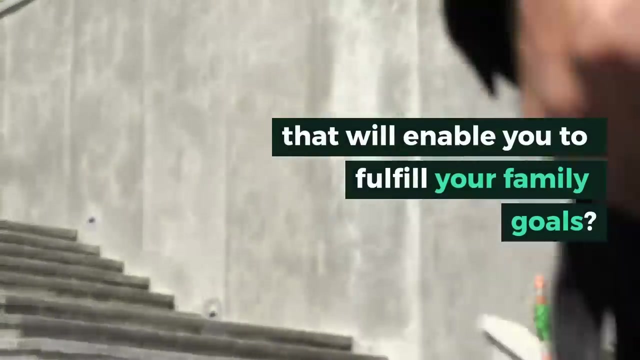 management and its major purpose. the second area of goals are your business and career goals. these are the how goals, the means by which you achieve your personal why goals. how can you achieve the level of income that will enable you to fill your family goals? how can you develop the skills and abilities to stay? 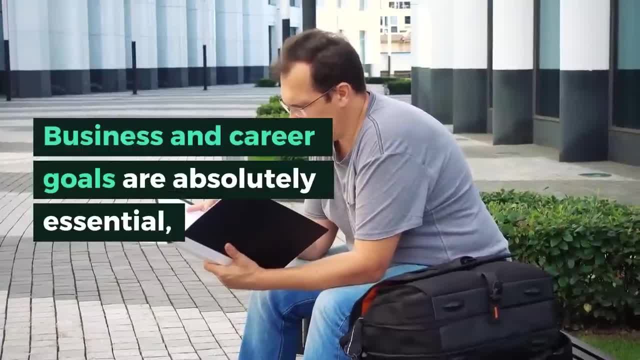 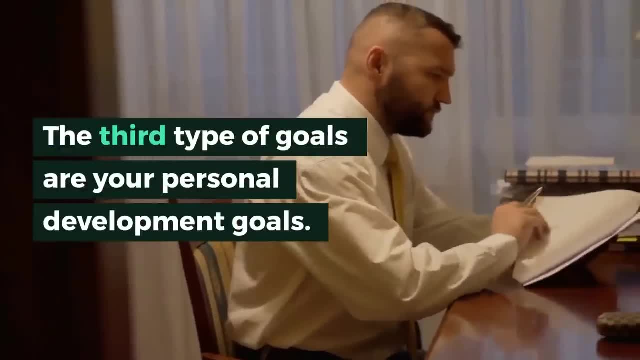 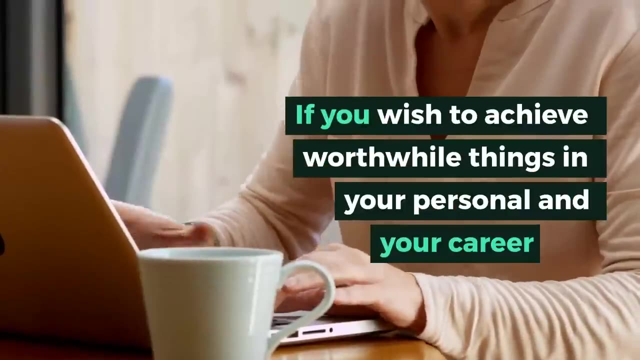 ahead of the curve in your career. business and career goals are absolutely essential, especially when balanced with family and personal goals. the third type of goals are your personal development goals. your outer life will be a reflection of your inner life. if you wish to achieve worthwhile things in. 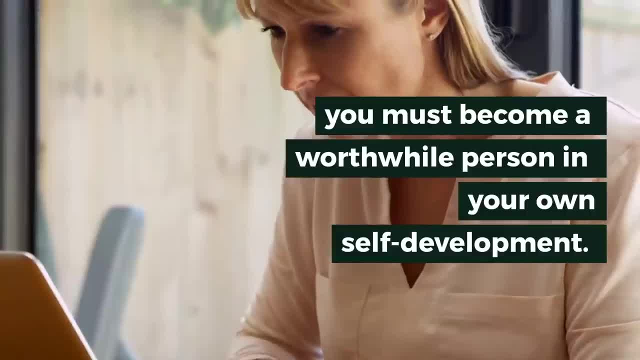 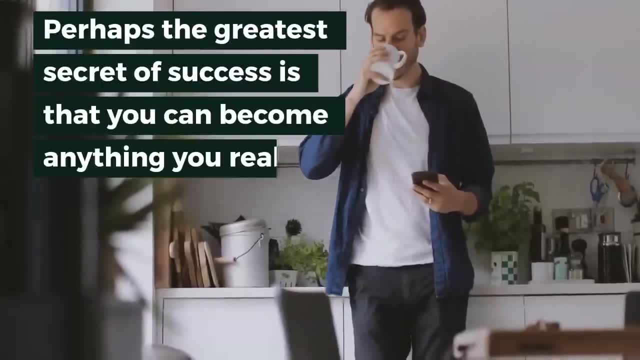 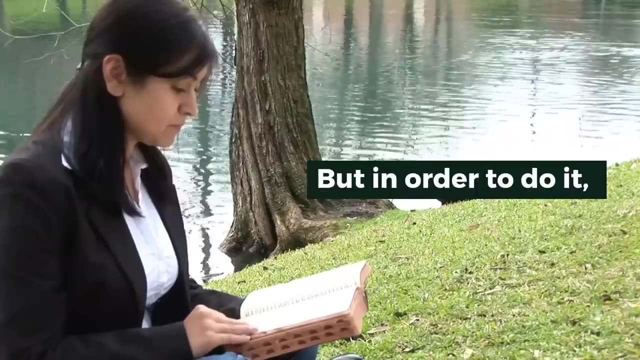 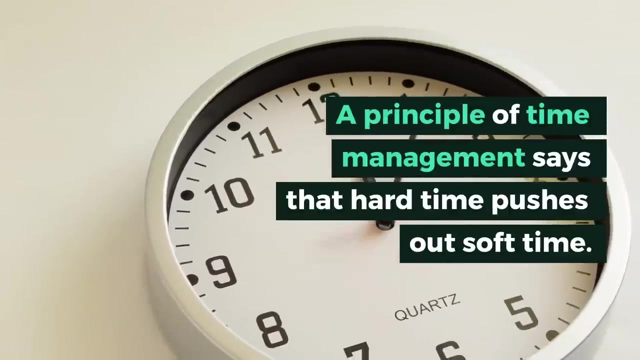 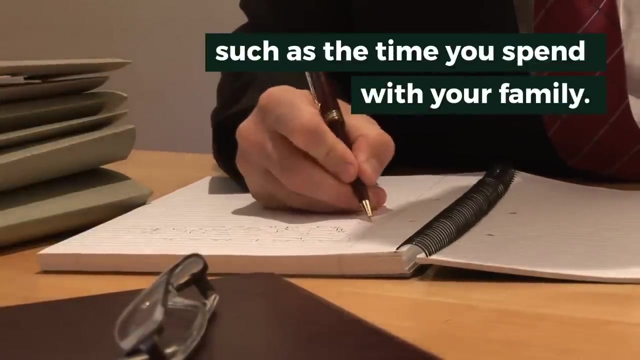 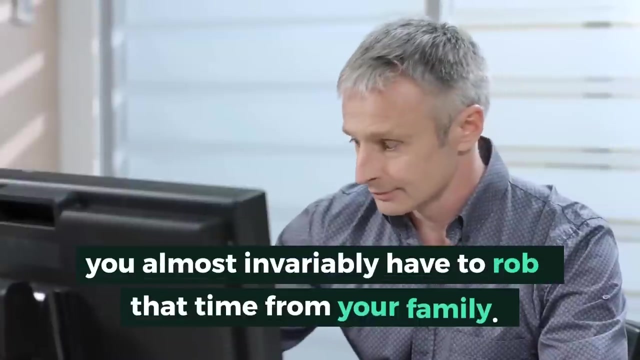 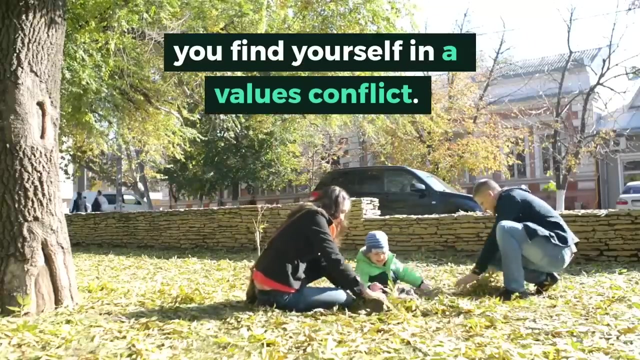 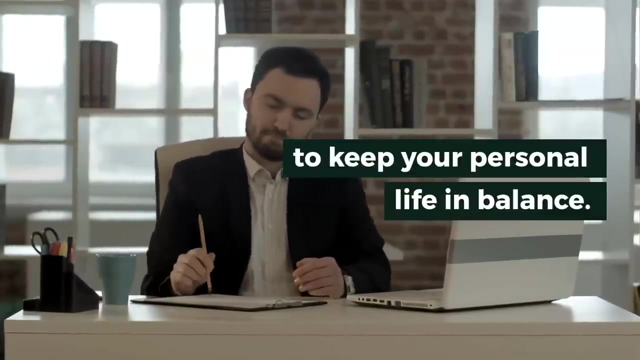 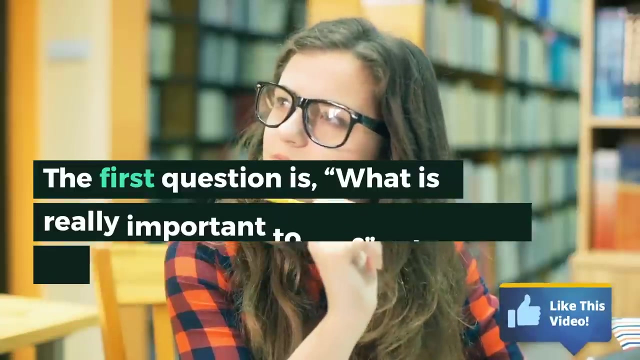 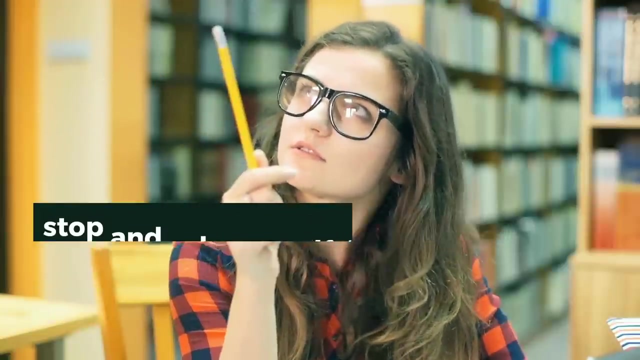 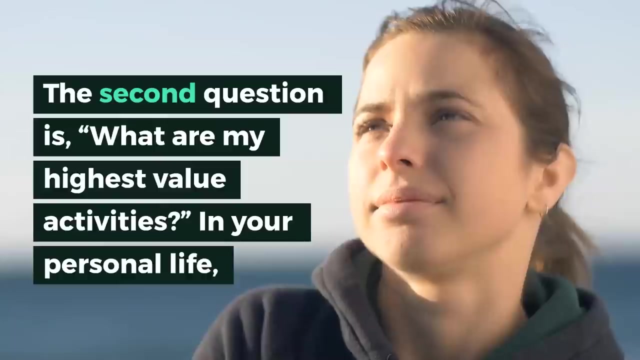 your personal and career life. you must become a worthwhile person in your own self development. you just need to know what you're doing, and what you're doing is the answer to that question. the second question is: what are my highest value activities in your personal life? this means, what are the things that I do that give me the